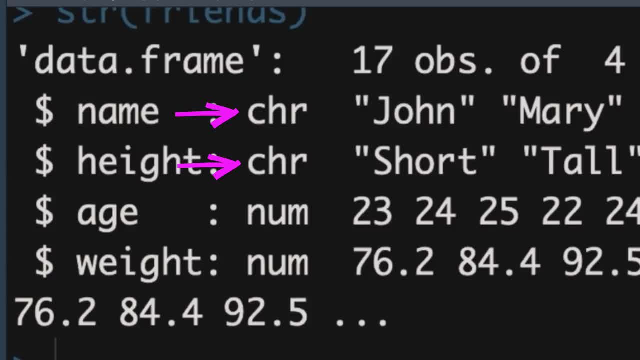 CHR, That's character. We're happy with that Height. it's called it a character, but we know that this is ordinal data. We want this to be called a factor, so we're going to change that. Age and weight are both called numerics. Now we said that numeric when R uses the term numeric. 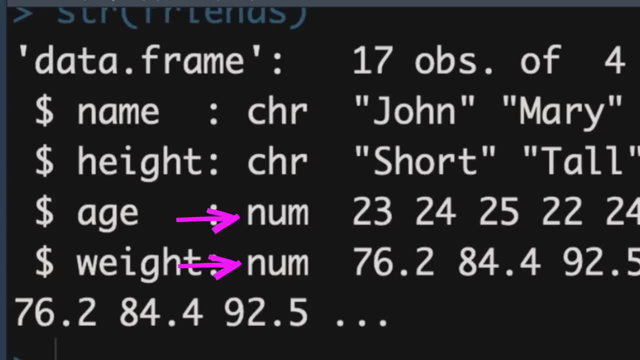 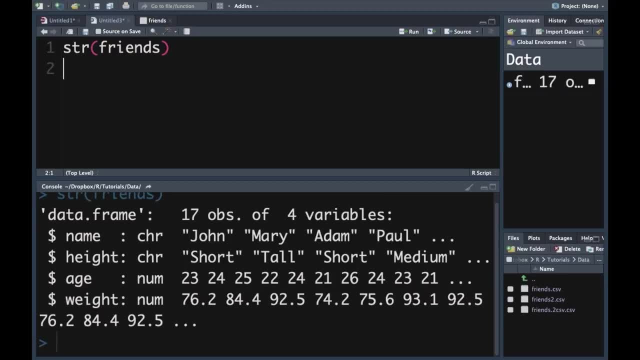 it means a continuous thought, a continuous variable. We want age to be an integer, Right? So wait, we're going to leave it numeric. Age, We're going to change to integer. So let's take a look at how to do that. To change the data type for the variable height from a character to a factor. 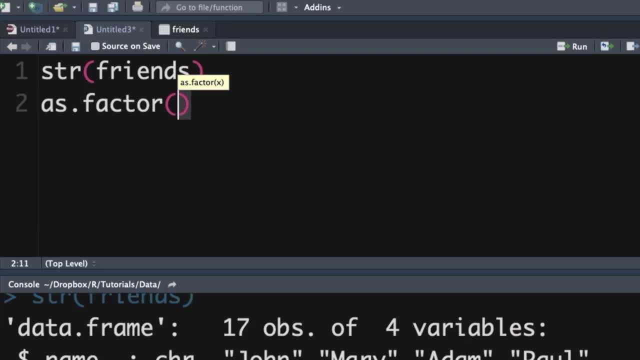 we use the command or the function as factor, right? And in the brackets we tell R what it should change, right? So we want to take. we want to take the data frame, friends, and within which we want to extract the variable height, and that line of code will do the trick, except we need to assign it to something, in other words, 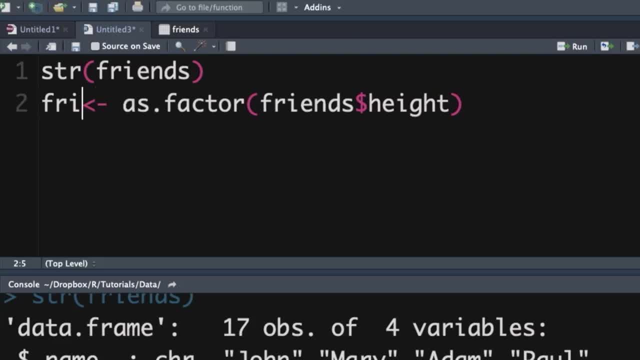 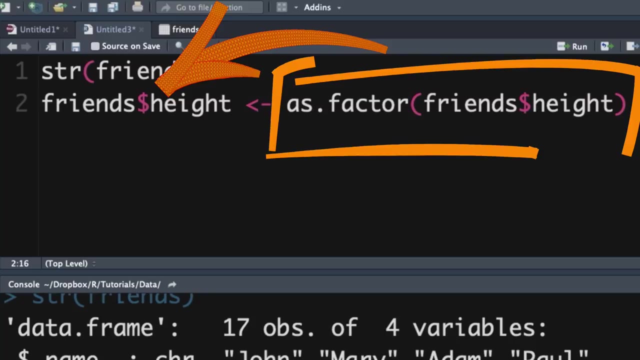 we put our little arrow over there and we say: friends, height. we're saying: assign all of this to the variable height in the data frame. friends, in other words, overwrite what is there at the moment. and if we push enter and rerun the first line of code asking for the 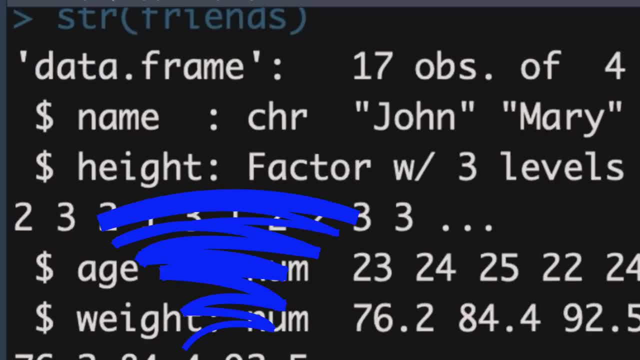 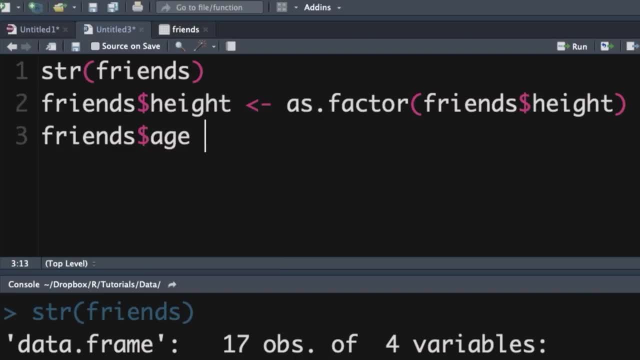 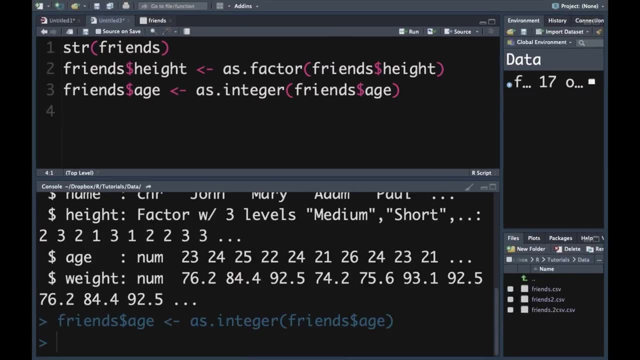 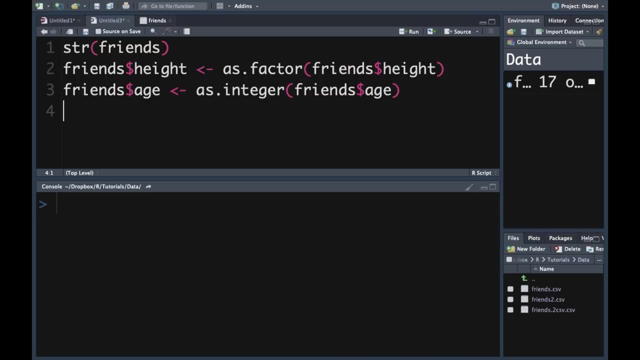 structure. we can see height is now a factor and similarly we can take the data frame friends, extract the variable age and we want to say as integer friends age, and that will change. let's run the first line of code again, age into an integer. so our variable height is a factor. that means it's a categorical ordinal variable. 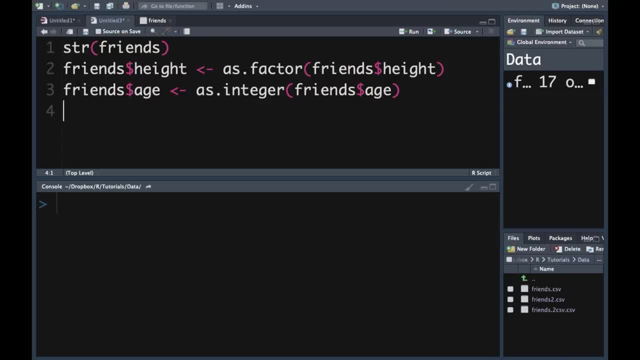 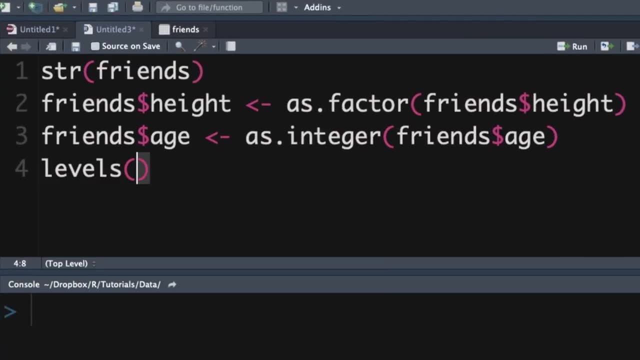 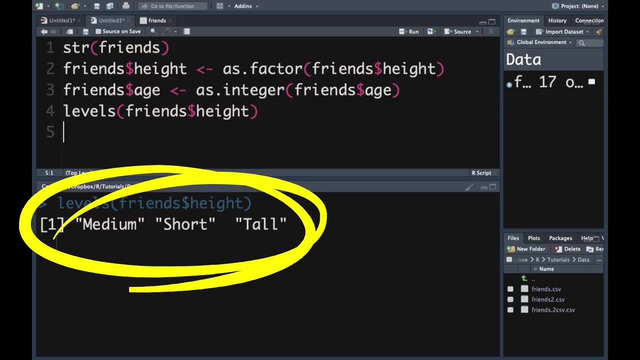 it's. it's a categorical variable where the categories have an order. okay, what order does our think the category should be in? well, we can ask our, we can say levels and friends, height, enter and in our console we'll see that r thinks a. It should be medium, short, tall. 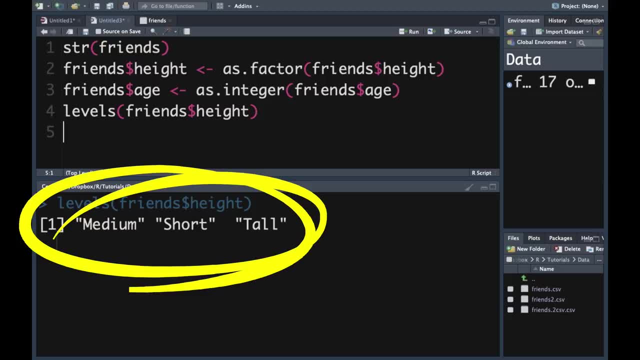 It's just stuck them in alphabetical order. We want it to be short, medium and tall, So let me show you how to make that change. So to change the levels of the height variable. this is what we do, all right. 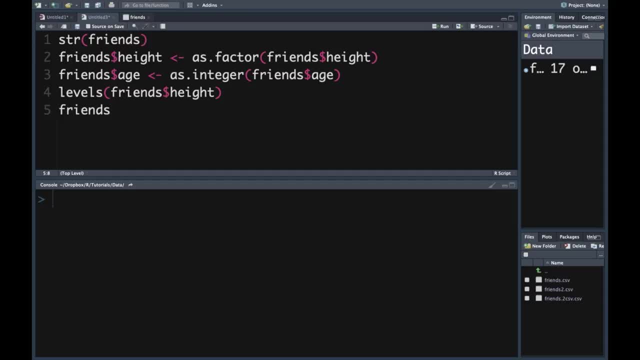 So again we start off with saying we're working with the dot frame, friends, We're working with the variable height, We're gonna assign to that. Now we don't say as factor, we say factor, all right. So leave out the as open brackets. 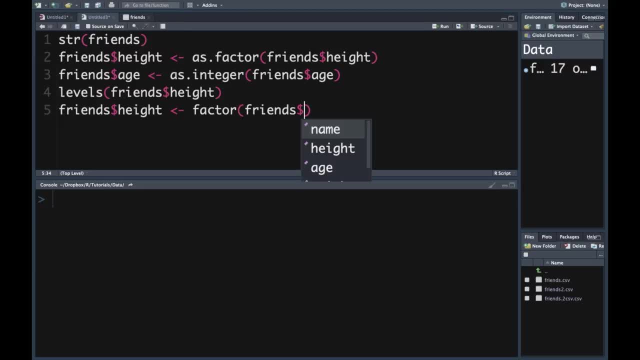 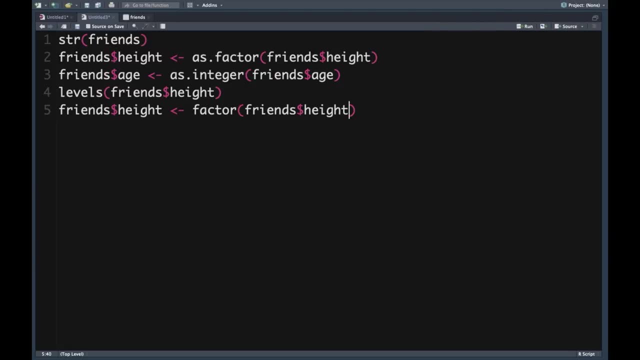 Again, tell it what you're working with Friends height. right Now we can say- and I'm actually gonna push shift control one just so that we zoom in on just the source, so you can see what I'm doing. all right, 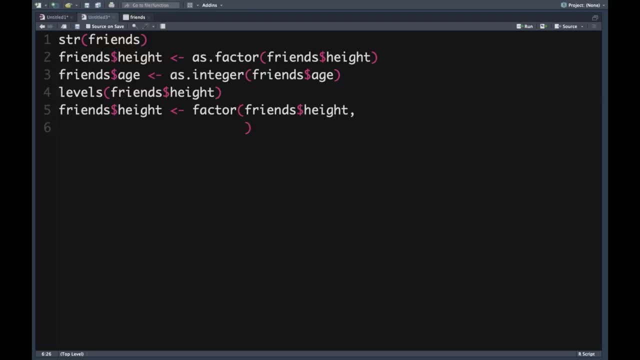 I'm gonna push a comma and I'm gonna push enter. Now R's just gonna continue to see this as one line of code. I'm just doing that so you can see what I'm doing. Now we're gonna say: levels equals C for concatenation. 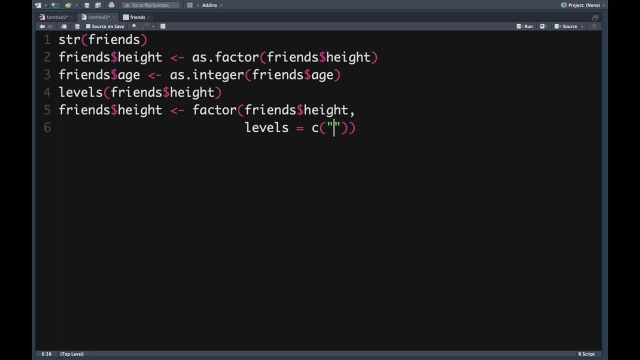 or combination of, and now we put in the order that we want them to be in. All right, so the C stands for concatenation and that just means whatever's in brackets, it needs to think of them together as one group And levels the word levels. there is just the second. 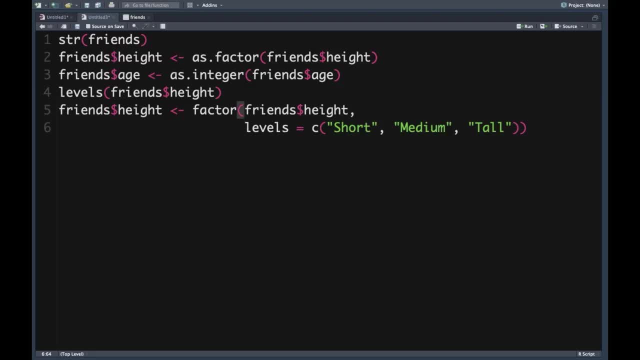 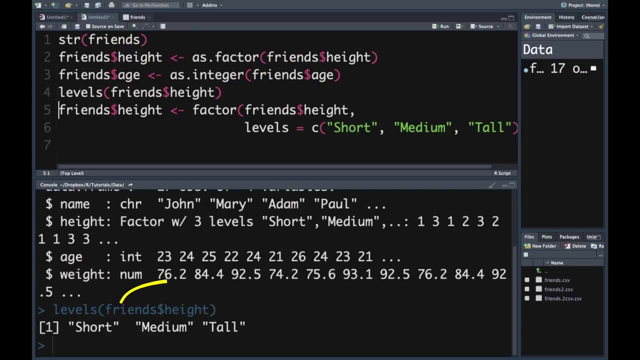 argument that gets applied in this particular instruction or associated with this particular function. Okay, I'm gonna push enter. If we rerun this line of code over here asking for the levels for that variable, we can see that they're short, medium and tall. 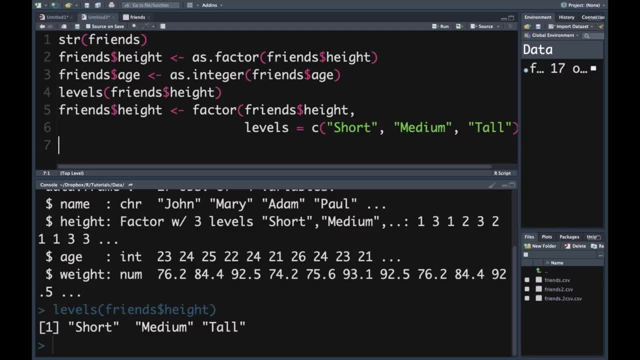 just the way we wanted them. So at the beginning of this video I said we're gonna talk about five kinds of variables, and so far we've only talked about four. The fifth kind of variable I wanna talk about is called a logical right. 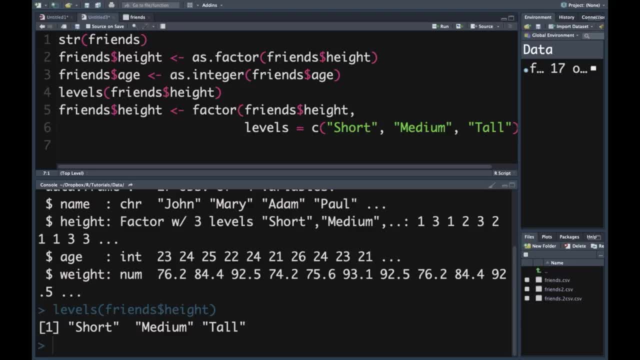 This is how a logical works. We can ask R a question of one of the other variables. right, These other variables? we think of them as something called a vector. A vector is a collection of data that's of the same type. So in our data frame we could ask R. 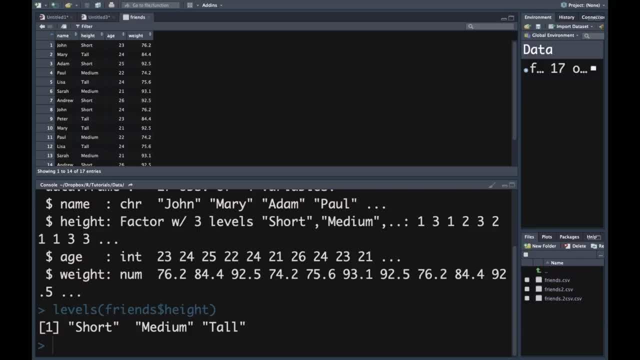 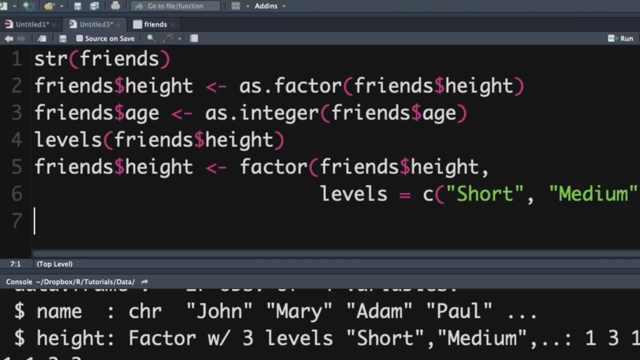 which of all of these people in our data frame, which of these are older than age 23?? And we could say we think of them as old, for example. right, So in our code over here we could say the age variable. 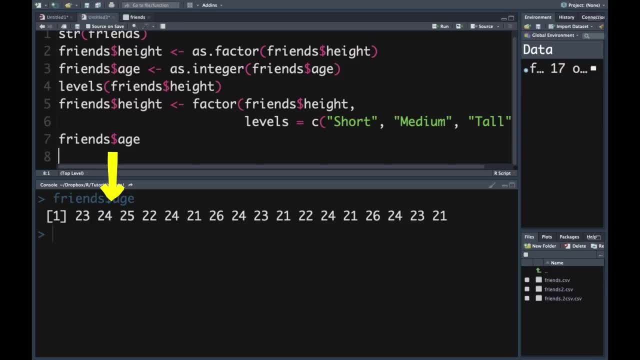 friends age and push command enter. we see in the console. we can see we call that a vector right. It's a collection of data of the same type. If we ask the question friends age and we said which of those are greater than 23,.